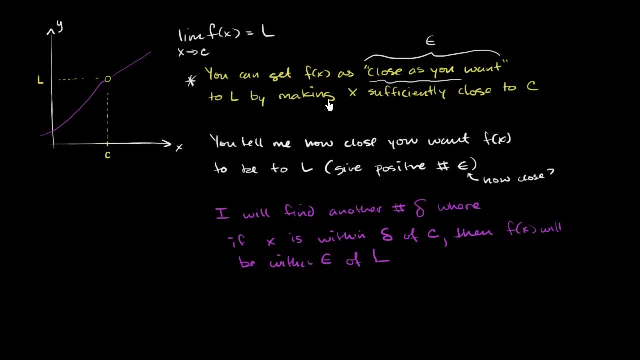 So let's see if these are really saying the same thing. In this yellow definition right over here we said: you can get f of x as close as you want to l by making x sufficiently close to c. This second definition which I kind of made- 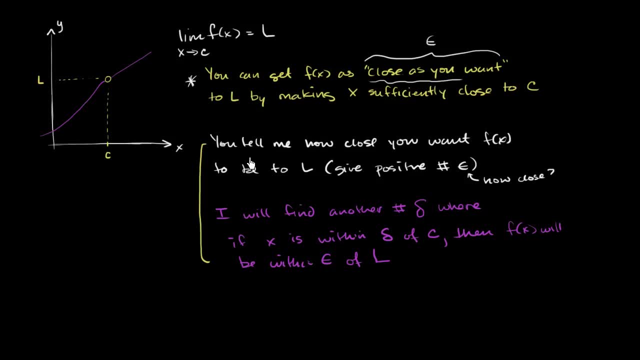 as a little bit more of a game is doing the same thing. Someone is saying how close they want f of x to b to l, And the burden is then to find a delta where, as long as x is within delta of c. 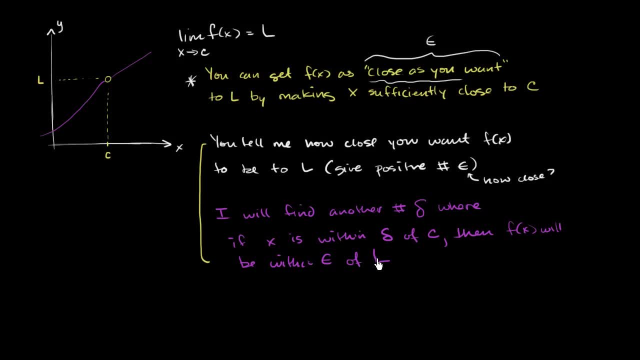 then f of x will be within epsilon of the limit. So that is doing it. It's saying: look, we're constraining x in such a way that if x is in that range to c, then f of x will be as close as you want. 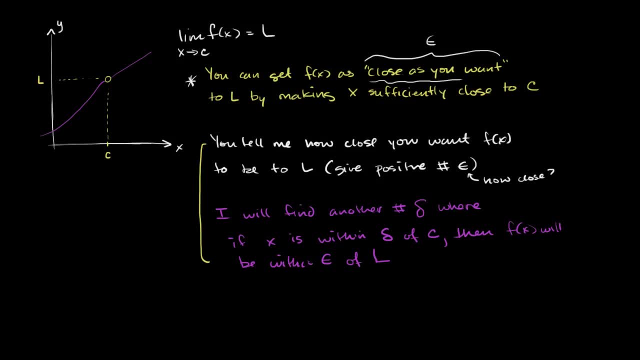 So let's make this a little bit clearer by diagramming. right over here You show up And you say: Well, I want f of x to be within epsilon of our limit. So this right over here, this point right over here, is our limit plus epsilon. 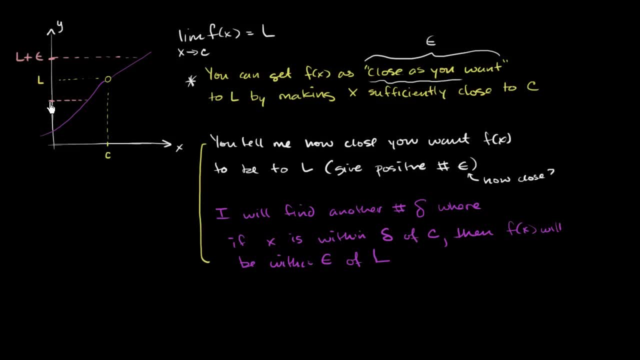 And this right over here might be our limit minus. This right over here is the limit minus epsilon. And you say, OK, sure, I think I can get your f of x within this range of our limit, And I can do that by defining a range around c. 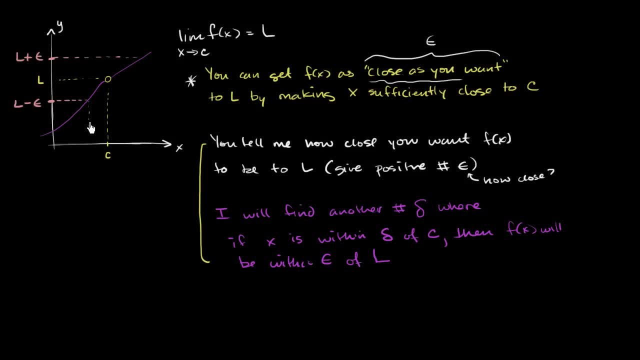 And really I could visually look at this boundary, But I could even go narrower than that boundary. I can go right over here. It says: OK, I meet your challenge, I will find another number delta. So this right over here is c plus delta. 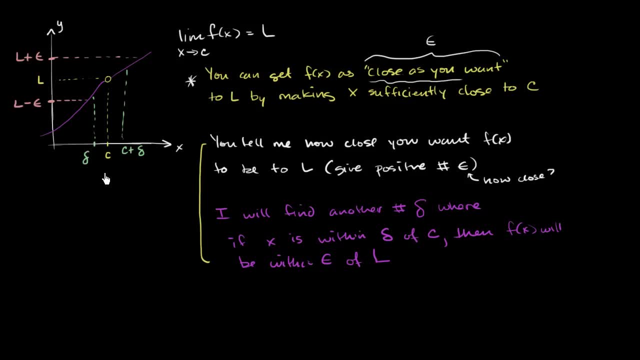 This right over here is c minus delta. So I'll find you some delta so that if you take each of these you'll get the same number. OK, If you take any x in the range c minus delta to c plus delta. 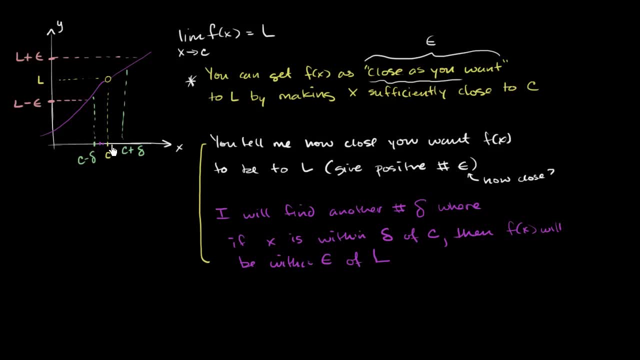 and maybe the function's not even defined at c. So we think of ones that maybe aren't c but are getting very close. If you find any x in that range, f of those x's are going to be as close as you want to your limit. 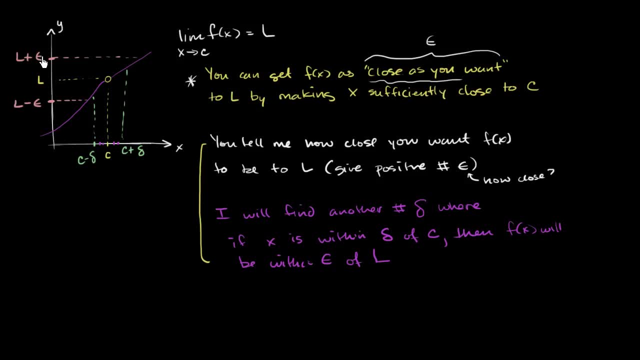 They're going to be within the range l plus epsilon or l minus epsilon. So what's another way of saying this? Another way of saying this is: you give me an epsilon, then I will find you a delta. So let me write this in a little bit more math notation. 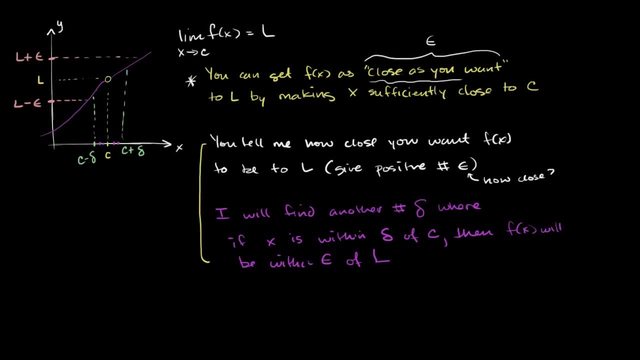 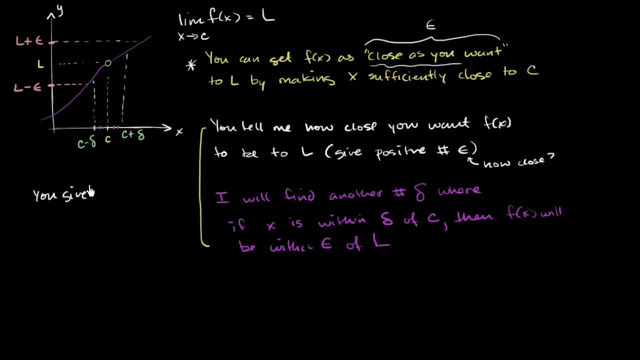 So I'll write the same exact statements, with a little bit more math here, but it's the exact same thing. So you give me, or let me write it this way: given an epsilon greater than 0.. OK, OK, OK. 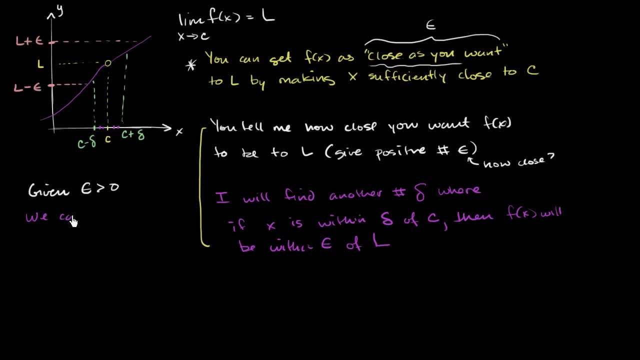 We can find- so that's kind of the first part of the game- we can find a delta greater than 0, such that if x is within delta of c. So what's another way of saying that x is within delta of c? Well, one way you could say: well. 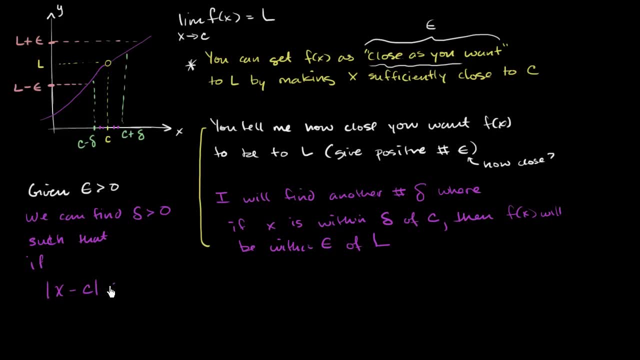 the distance between x and c is going to be less than delta. This statement is true for any x that's within delta of c. The difference between the two is going to be less than delta, So that if you pick an x that is in this range between c. 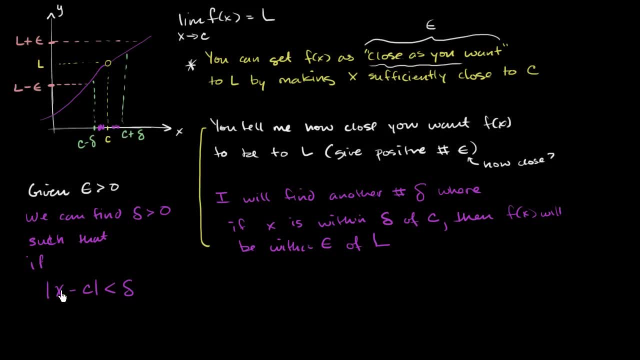 minus delta and c plus delta, and these are the x's that satisfy that right over here. then- and I'll do this in a new color- then the distance between your f of x and your limit, and this is just the distance between the f. 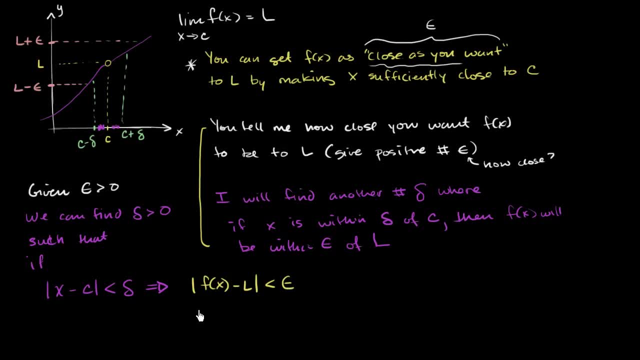 of x and the limit, it's going to be less than epsilon. So all this is saying is, if the limit truly does exist- it truly is- l is, if you give me any positive number, epsilon, it could be a super, super small one. we can find a delta. 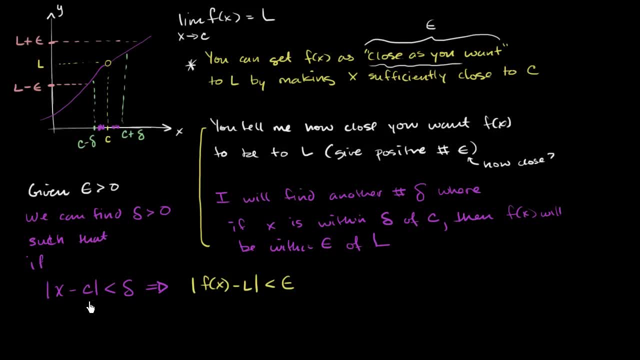 So we can define a range around c, So that if we take any x value, that is within delta of c. that's all. this statement is saying that the distance between x and c is less than delta, So it's within delta c. 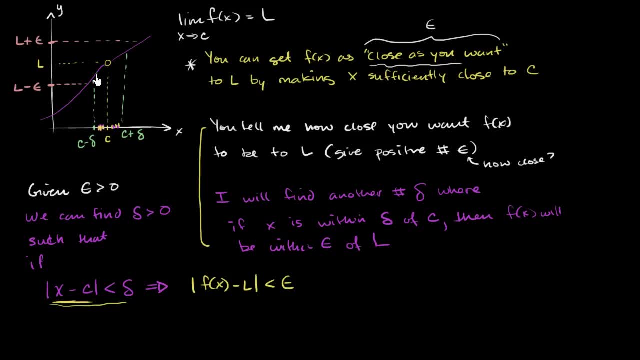 So that's at these points right over here, That f of those x's, that f of the function evaluated at those x's is going to be within the range that you are specifying. It's going to be within epsilon of our limit. 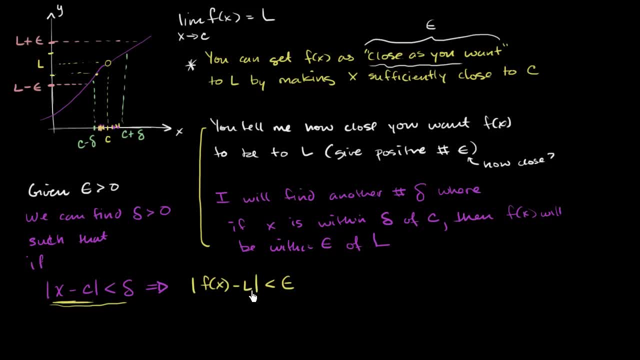 The f of x. the difference between f of x and your limit will be less than epsilon. Your f of x is going to sit someplace over there. So that's all the epsilon delta definition is telling us. In the next video we will prove.